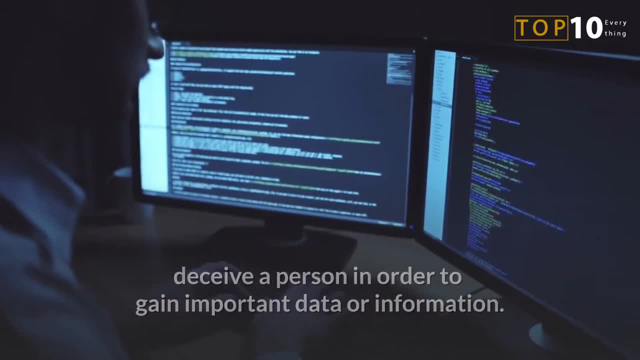 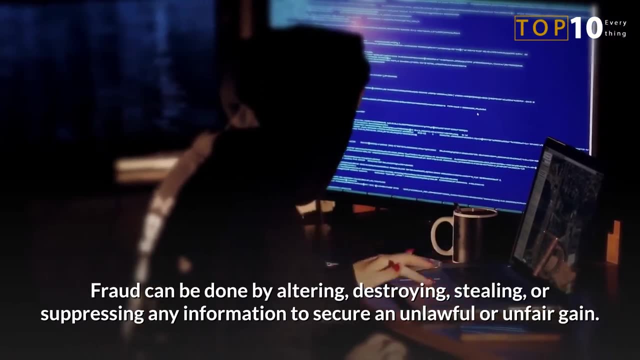 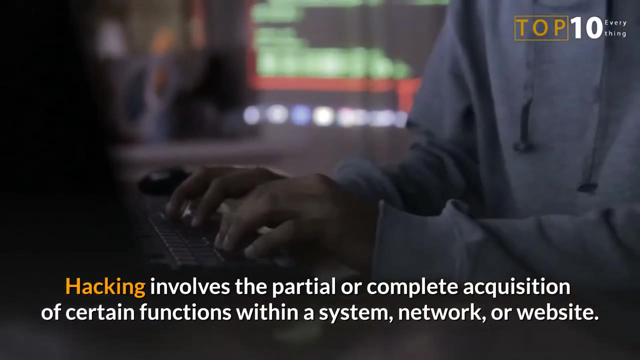 in order to gain important data or information. Fraud can be done by altering, destroying, stealing or suppressing any information to secure an unlawful or unfair gain. 9. Hacking: Hacking involves the partial or complete acquisition of certain functions within a system, network or website. It also aims to access to important 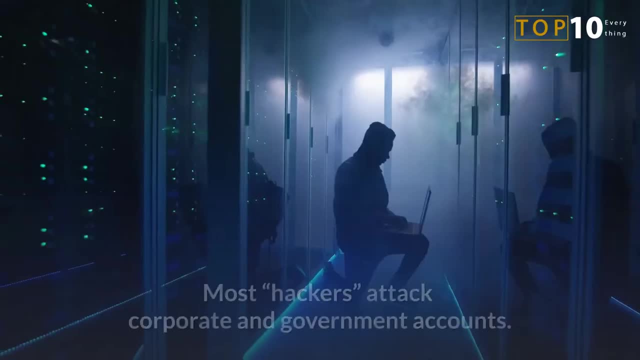 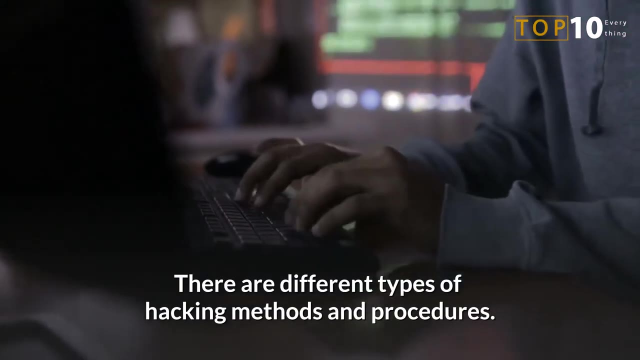 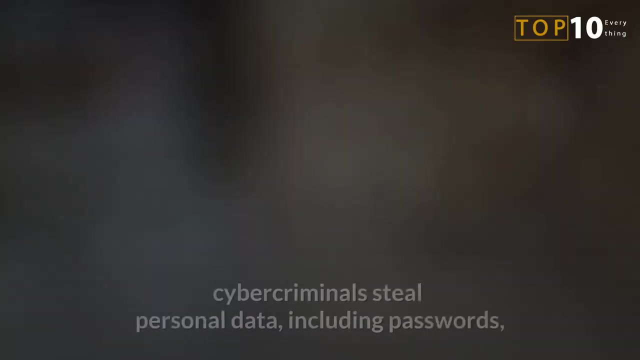 data and information breaching privacy. Most hackers attack corporate and government accounts. There are different types of hacking methods and procedures. 8. Identity Theft. Identity theft is a specific form of fraud in which cybercriminals steal personal data, including passwords, data about the bank account. 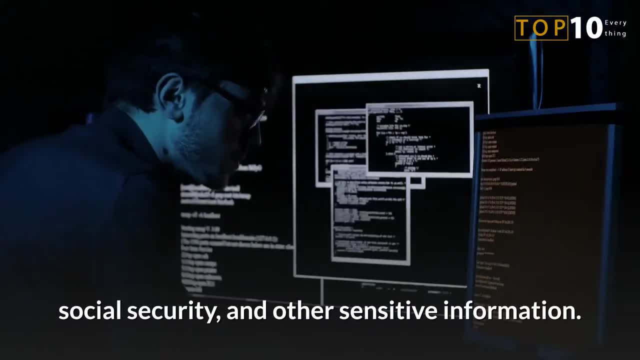 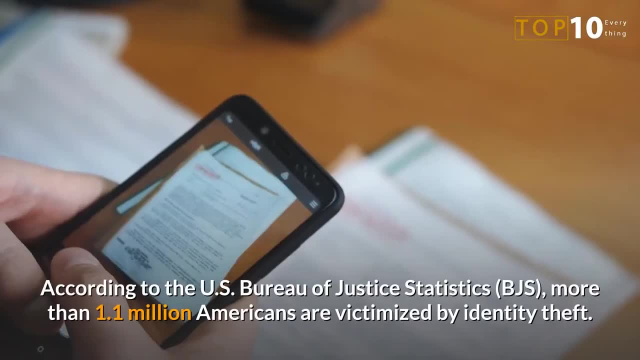 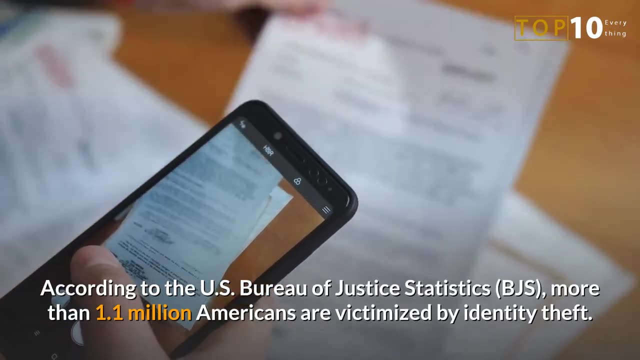 credit cards, debit cards, social security and other sensitive information. Through identity theft, criminals can steal money. According to the US Bureau of Justice Statistics, more than 1.1 million Americans are victimized by identity theft. 7. Scamming: 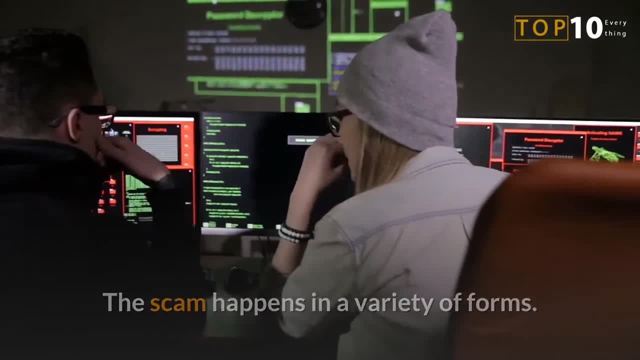 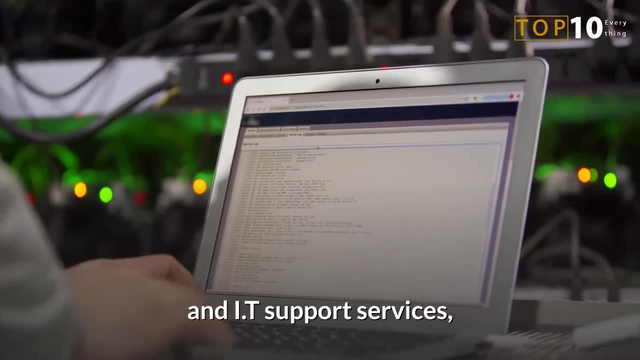 The scam happens in a variety of forms. In cyberspace. scamming can be done by offering computer repair, network troubleshooting and cybercrime protection- In the United States, network troubleshooting and IT support services, forcing users to shell out hundreds of money for cyber problems that do not even exist. 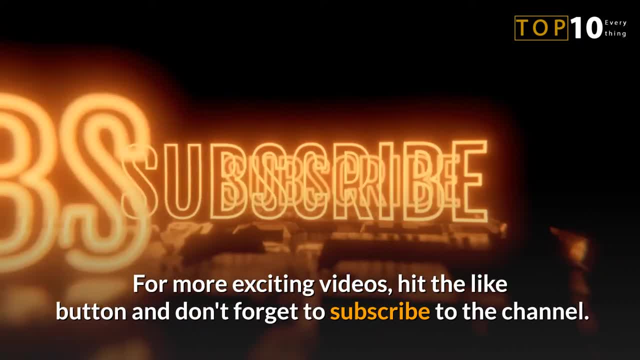 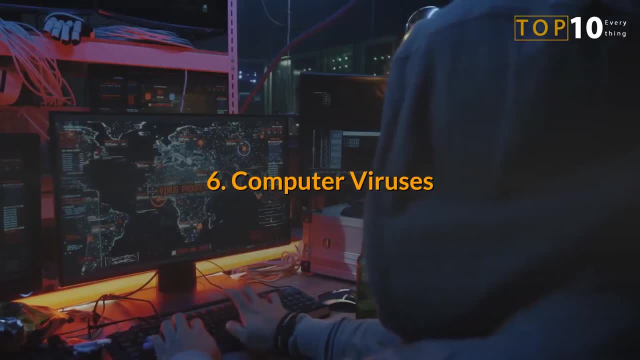 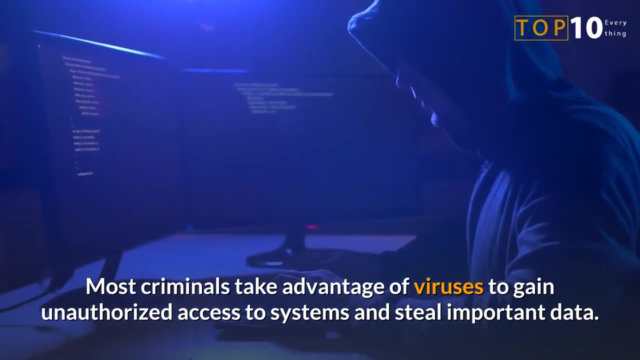 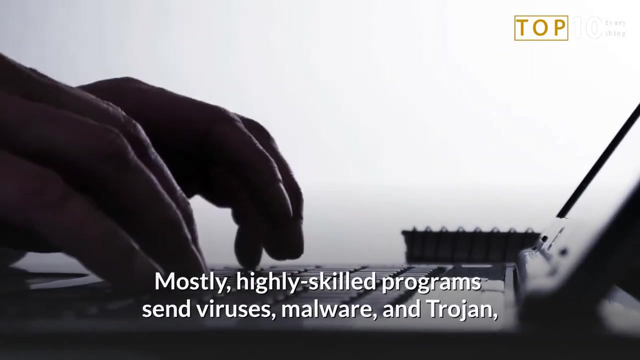 For more exciting videos, hit the like button and don't forget to subscribe to the channel. Any Illegal Plans to Make Money Fall to Scams. 6. Computer Viruses. Most criminals take advantage of viruses to gain unauthorized access to systems and steal important data. Mostly highly skilled programs send viruses, malware and Trojan. 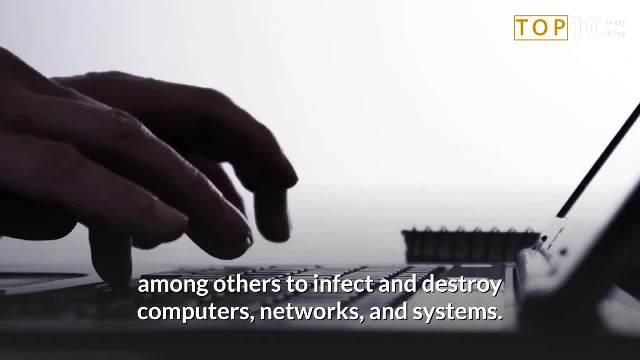 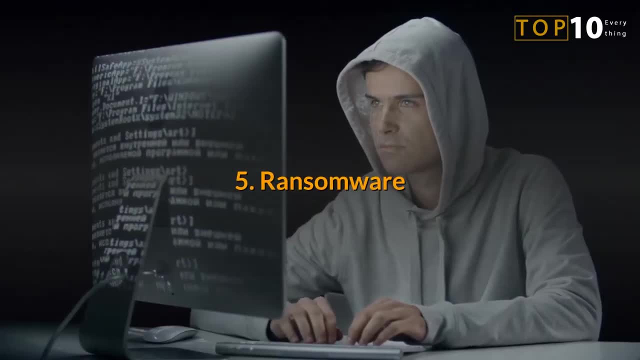 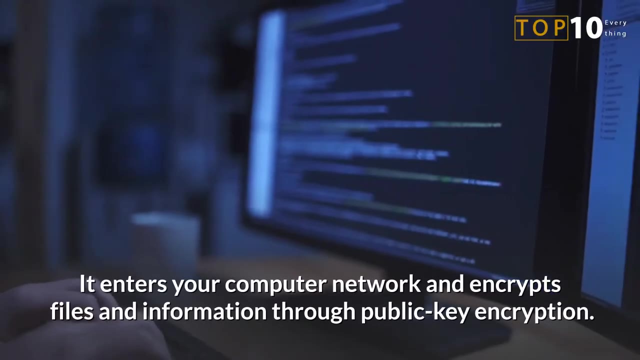 among others, to infect and destroy computers, networks and systems. Viruses can spread through removable devices and the internet. 5. Ransomware: Ransomware is one of the most destructive malware-based attacks. It enters your computer network and encrypts files and information through public key encryption.